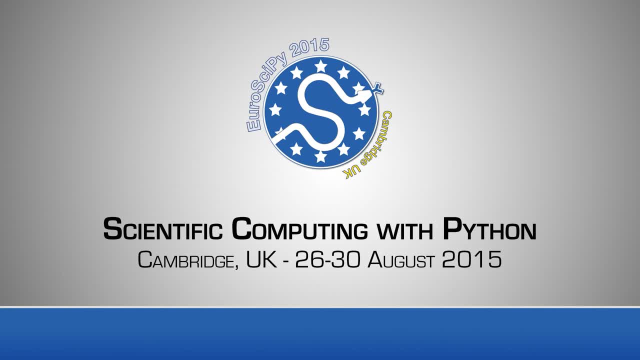 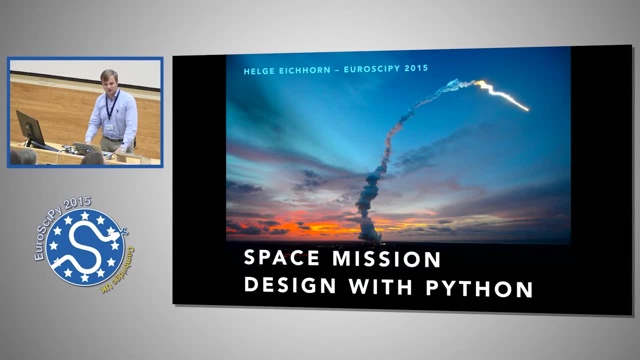 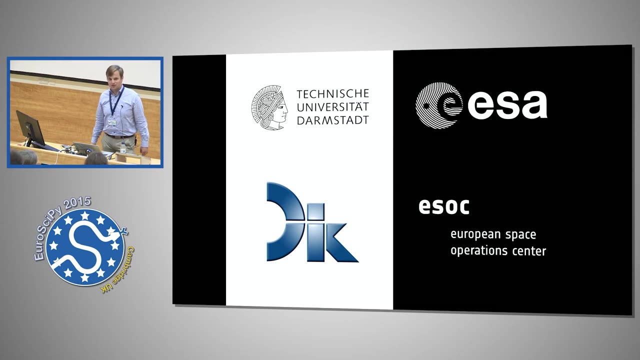 All right, so welcome to space mission design with Python, And my name is Helge Eichhorn, and by day I'm a PhD student at Technische Universität Darmstadt, where I do research in model-based engineering, and at the Department of Computer Integrated Design. 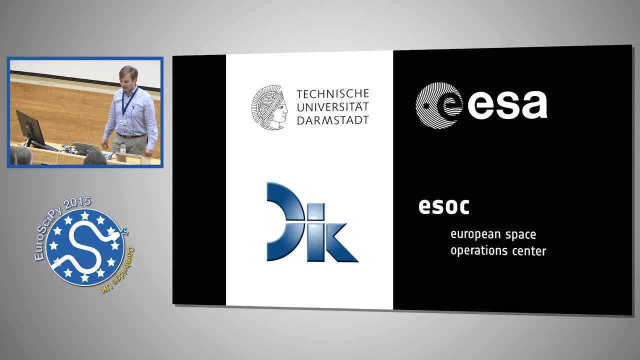 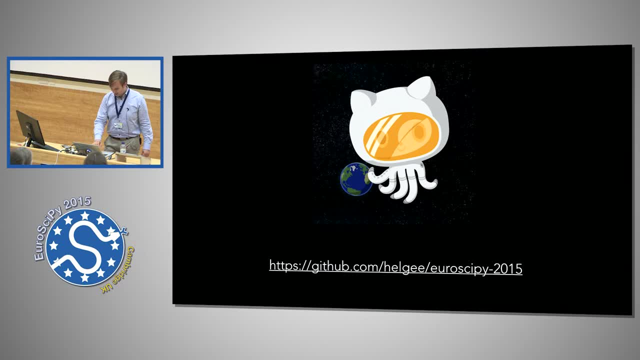 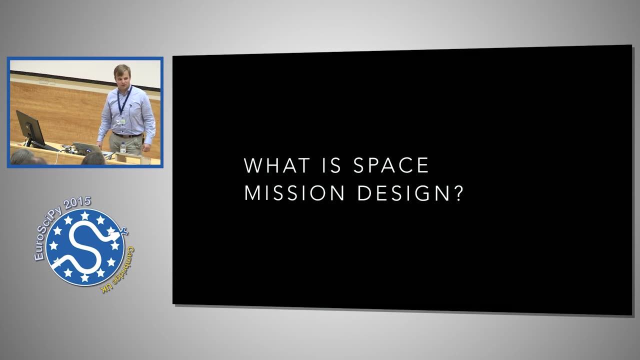 By night. on the other hand, I support the mission analysis section at the European Space Operations Center as an external consultant And I'm Helge on GitHub. So the first question is: what is space mission design? So we could also speak about trajectory design. So it is about determining how a spacecraft will reach its target orbit, and that efficiently, in a reasonable amount of time, without violating any engineering constraints, and it should also fulfill all the scientific objectives on the way. 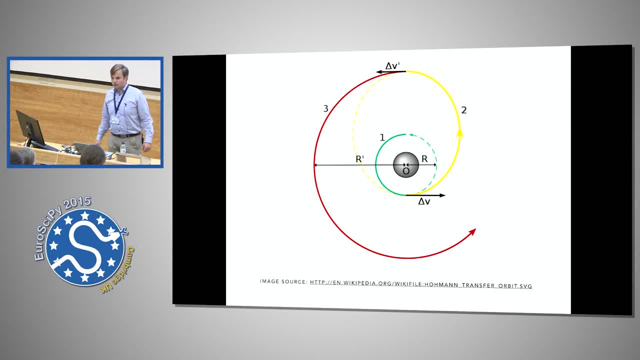 So what you need to do is you need to model the orbit of the spacecraft and then optimize to find the best possible trajectory. But the point is, since every scientific space mission and spacecraft are unique and the engineering design is tightly coupled with the mission design, you need to iterate a lot during the development of the mission and you need to be able to answer a lot of questions. 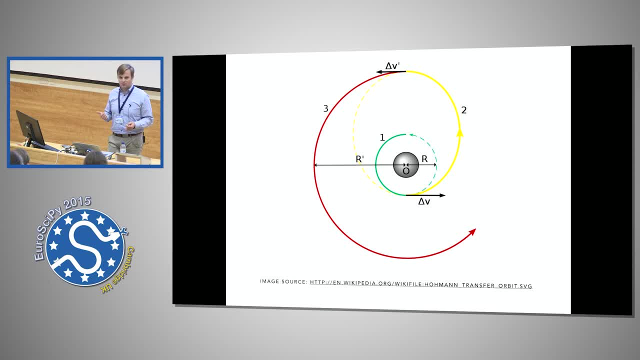 And you need to be able to answer a lot of questions, And that's fast. So will there be eclipses, So will the spacecraft enter the shadow of the Earth, How hot will it get? How much station keeping? So how much fuel do we need to keep the spacecraft in orbit? 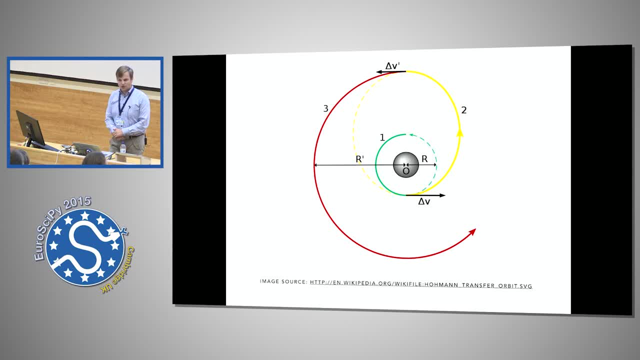 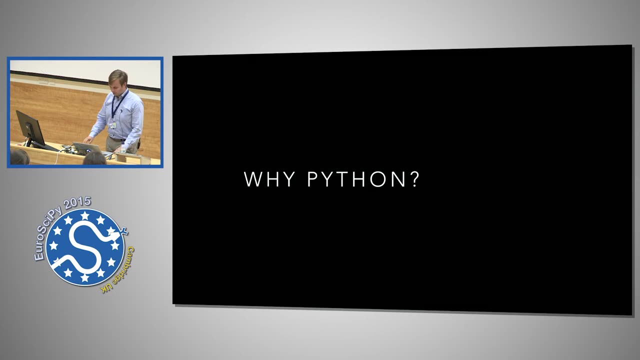 And the task is quite computation heavy. So the gold standard has been FORTRAN and MATLAB for visualization. So then why Python? So at the mission analysis section at the European Space Operations Center there's a large body of very well-tested FORTRAN-77 code. 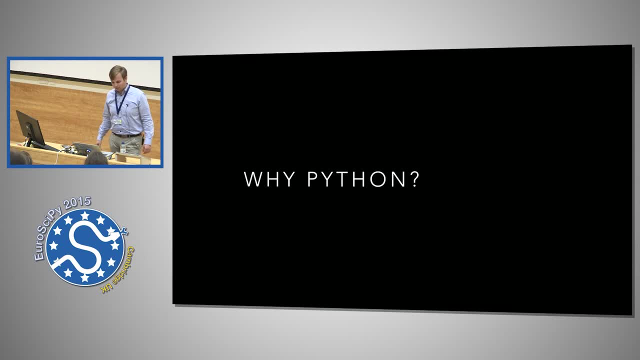 And of course, as it is usual with FORTRAN-77, it's very dense and cryptic and the barrier of entry for newcomers is tremendously high. So my fellow trainees and I were swearing a lot. And the other problem with FORTRAN-77 is that if your only tool is a handgun, 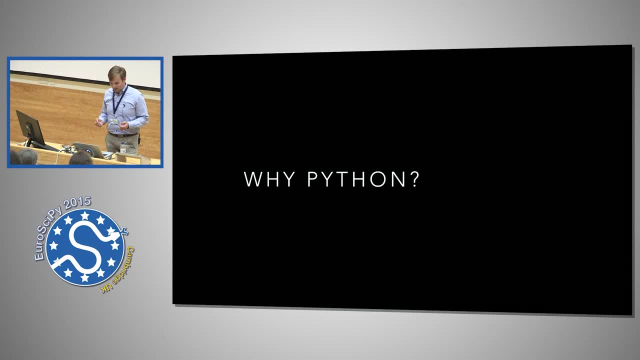 and you use a sledgehammer, every problem starts to look like a nail. And I must say FORTRAN-77 is probably the most beautiful and most awesome sledgehammer in existence. You can do too much with it for your own good. 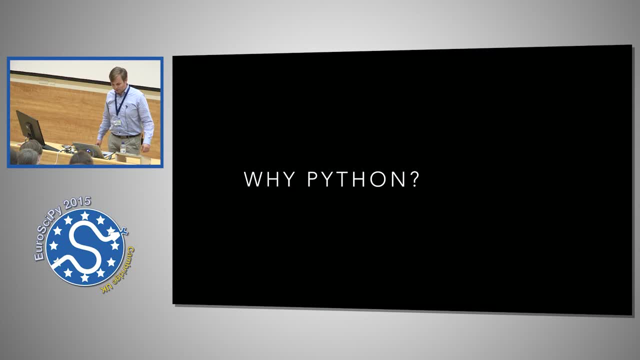 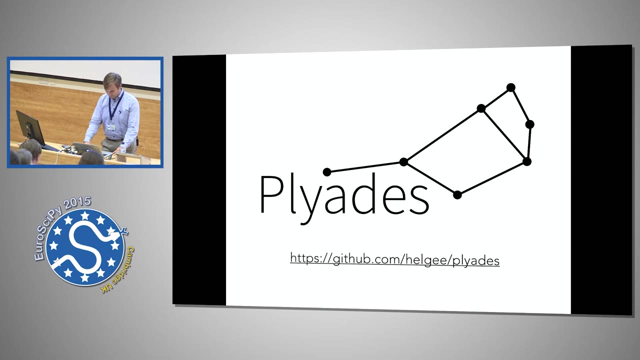 So I think I'm probably preaching to the choir when I say that if you want to start saving brain cycles instead of CPU cycles, we need better tools and better APIs and better abstractions, hence Python. So during one very nasty fight with the compiler, I did what every good scientist does when deadlines are looming. 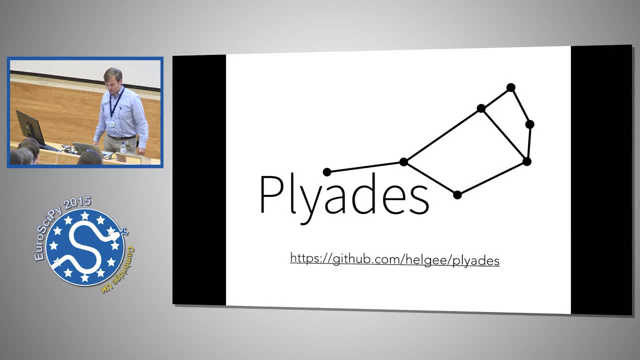 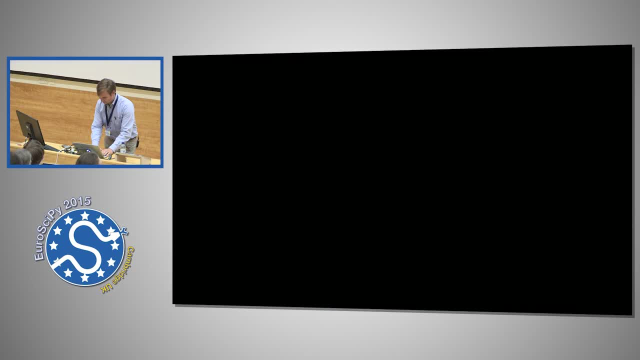 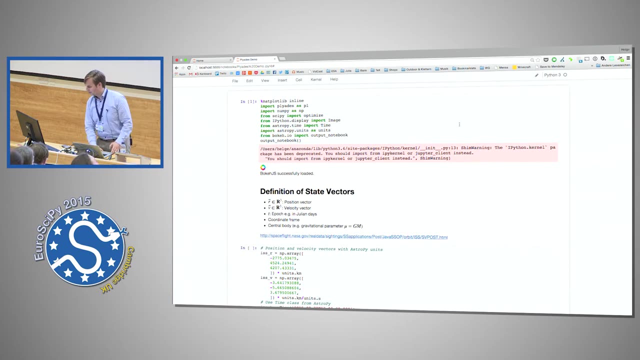 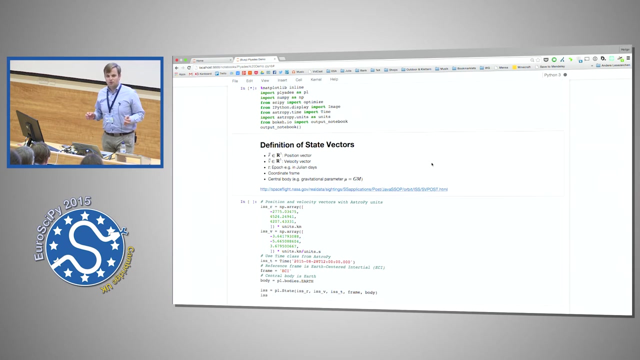 I started my very own open-source project, Pleiades, a Python pseudodynamics library which I would like to present to you. now. There's the cursor, All right. So what I wanted to do here was to rethink the basic building blocks. 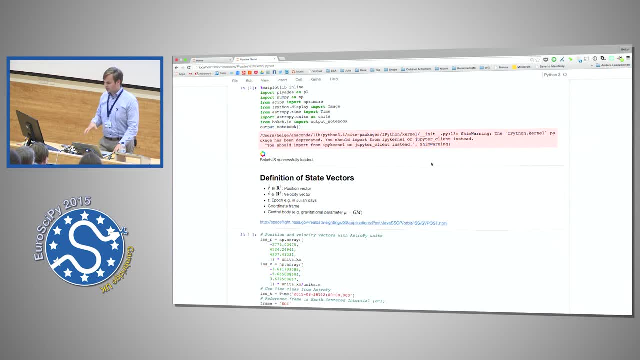 So what is the first thing we need to determine the state of a spacecraft? It's a state vector. So we have a position vector in three-dimensional space, We have a velocity vector in three-dimensional space, We have the point in time for the state vector, a coordinate frame and a central body with certain parameters. 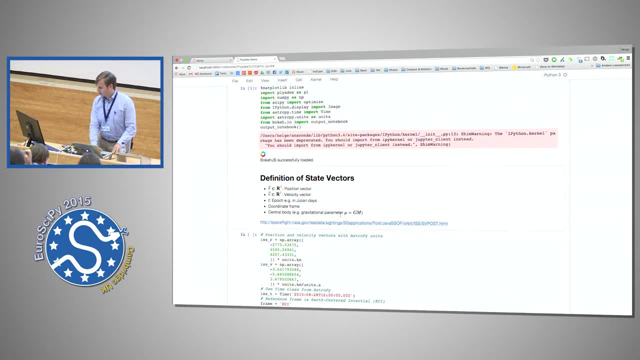 For example, the gravitational parameter, which is the gravitational constant times the mass of the central body. So what would be the Fortran 77 approach? Well, the first three we dump in a seven-element double array. That is of course part of the variable name. 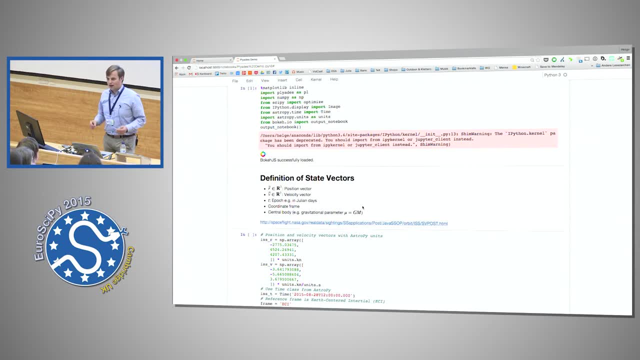 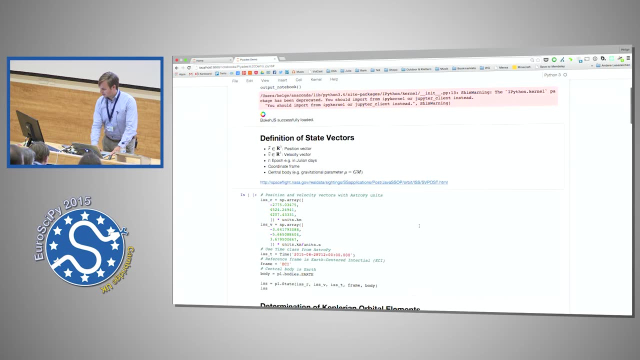 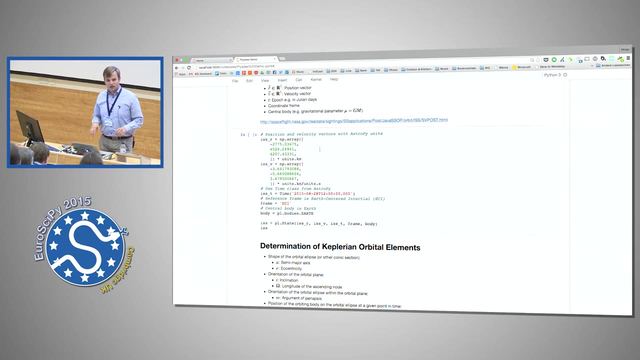 And this is a common block somewhere, And I am lazy, I don't want to keep that all in my head. So what I did is I wrote a new state vector class, And what we want to do now is do a little analysis. 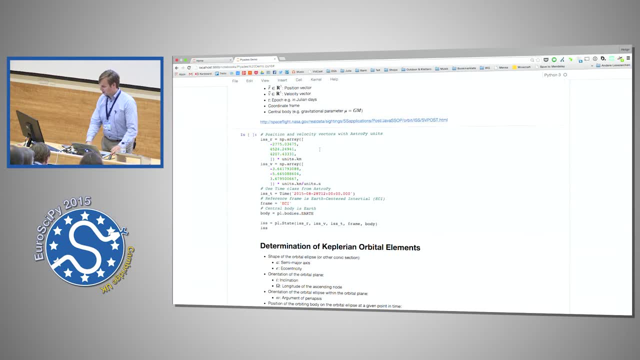 So we do some predictions about the orbit of the ISS. So this is the position vector in kilometers. I'm using astropy units, which is really nice, Unless you run into problems then it's nasty- And the velocity vector. again, a time object from astropy. 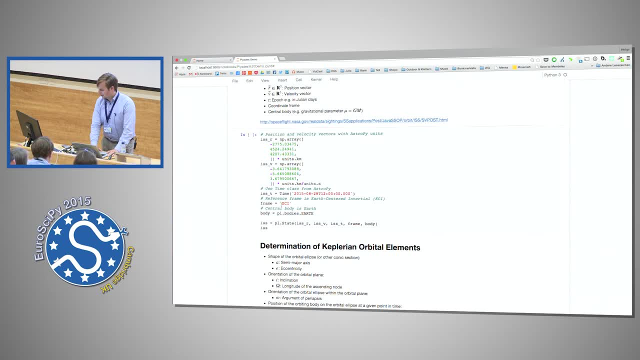 which is also really nice- The coordinate frame and the central body That is the Earth, And now we construct a state object And pretty printed in the notebook. So there's a lot of stuff here, And so what can we tell about the properties of the orbit from this? 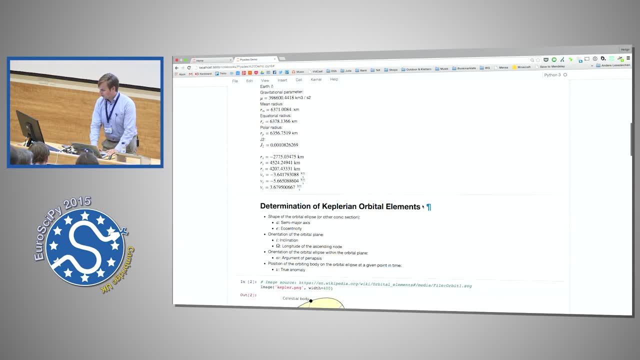 Exactly nothing at all. So we need some more information. So what? The first thing you do to determine how the orbit looks like is to calculate the Keplerian or classical orbital elements. So we want to describe the shape of the orbital ellipse. For that we need the semi-major axis and the eccentricity. 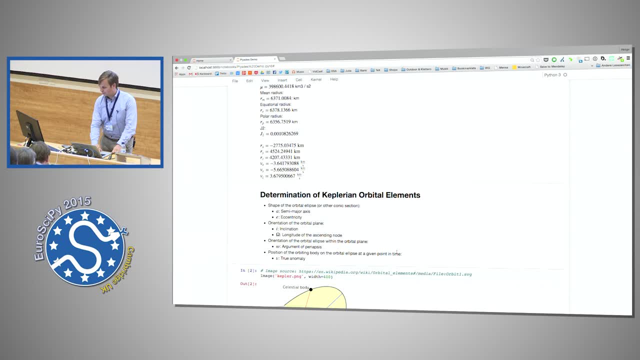 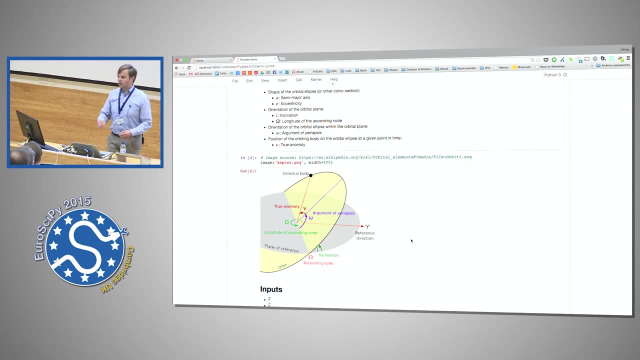 So how oval the ellipse is. Then a few angles, And I have a picture here. So the inclination, which is the angle between the plane of reference and the orbital plane, The longitude of the ascending node, Which is the angle between the reference direction. 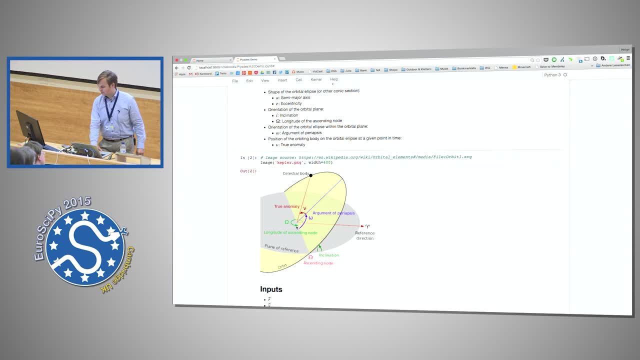 and the node line which is the intersection of the two planes, So how the orbit is located or is rotated towards the reference direction. Then we need to determine the orientation of the orbital plane. So we have the orbital ellipse within the orbital plane. 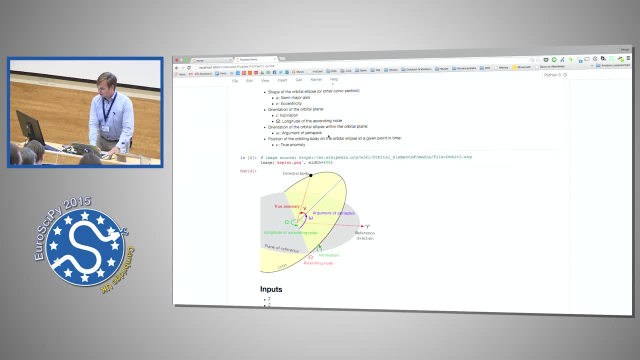 And that's the so-called argument of periapsis. And lastly, we need to know the position of the orbiting body on the orbital ellipse, And that's the so-called true anomaly. What do we need as inputs? We need the position vector and the velocity vector. 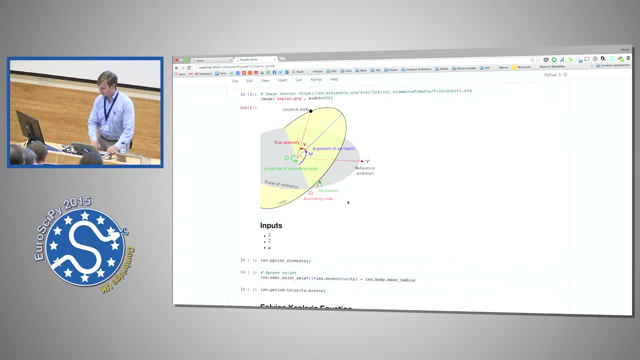 and the gravitational parameter. And nice, we have all of that, So we can directly calculate it and print it. So we see, the eccentricity is close to zero, which means the orbit is almost circular And the inclination is below 180 degrees. 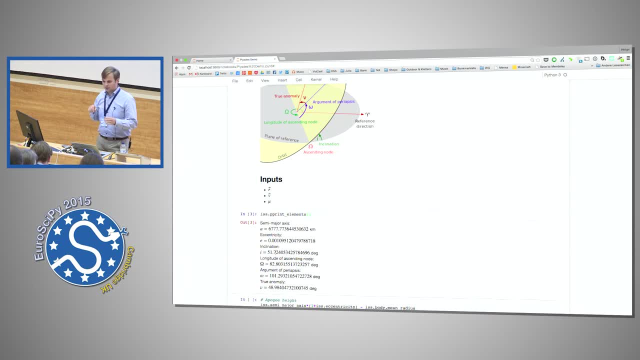 That means it's a pro-grade orbit, So the sense of rotational direction is the same as the orbits of the Earth, And we can derive some other quantities from that. So the apogee height of the ISS is 414 kilometers right now. 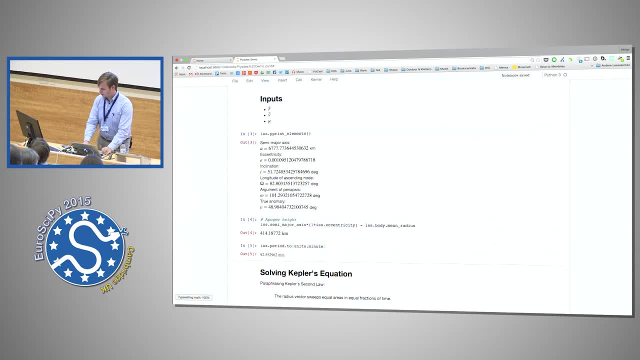 And the orbital period is 92 minutes. So the ISS circles the Earth in 90 minutes. So now the next step is: we want to predict the orbits sometime in the future. So what we need to do here is some math and solve Kepler's equation. 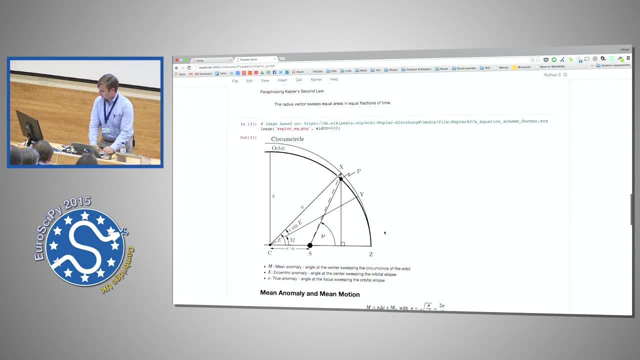 So we can determine. we need three angles here. So what we're interested in is this one, the true anomaly, So the point at which the spacecraft is on the orbit. And there's two more. There is the mean anomaly, which is the angle at the center of the ellipse. 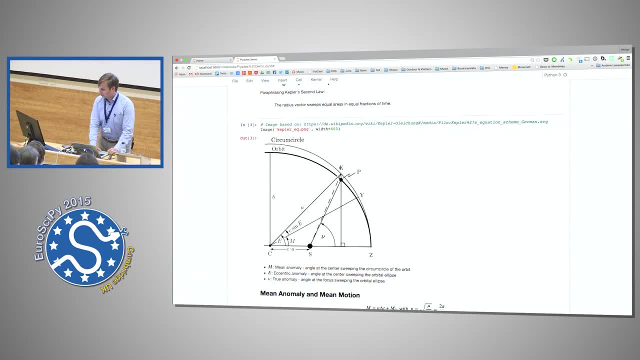 which sweeps the circumcircle Sounds complicated. I will tell you why we need that. And the eccentric anomaly which is also at the center and sweeping the orbital ellipse. And the good thing about the mean anomaly is that it increases linearly with time. 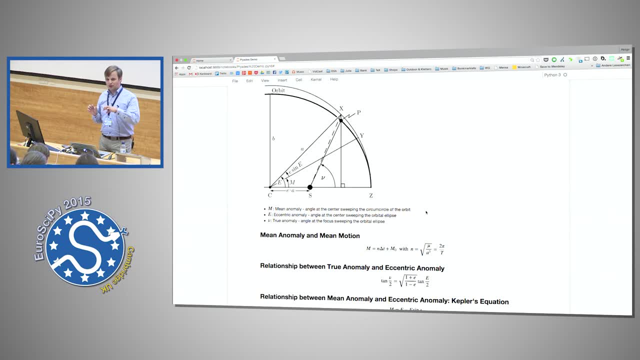 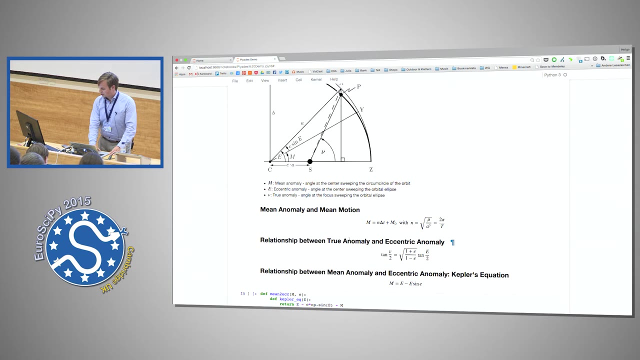 So on the ellipse the other two angles, so the angular velocity is changing. But with the delta t we can directly determine the mean anomaly And there's a relationship between the true anomaly and the eccentric anomaly. And then there is a relationship 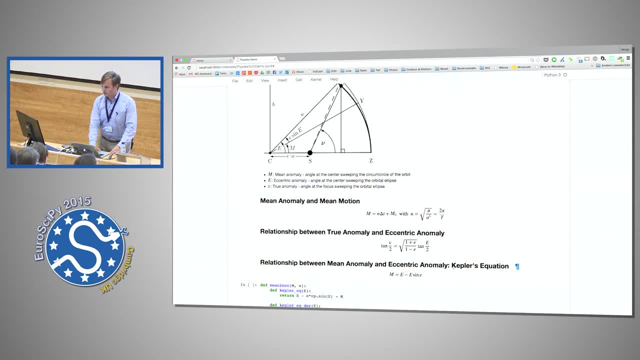 between the mean anomaly and the eccentric anomaly, which is Kepler's equation. And now we're screwed, because we can solve that analytically, Except we're not because Python to the rescue. we use the Newton-Raphson method from SciPy. 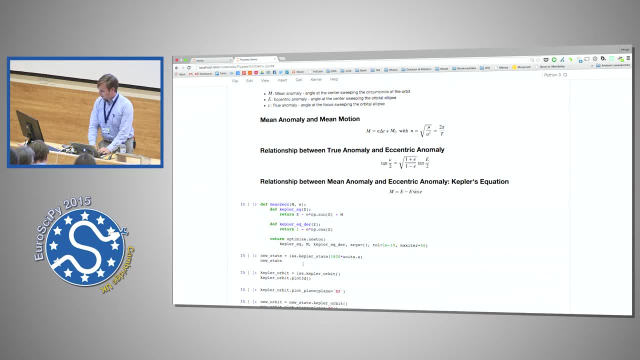 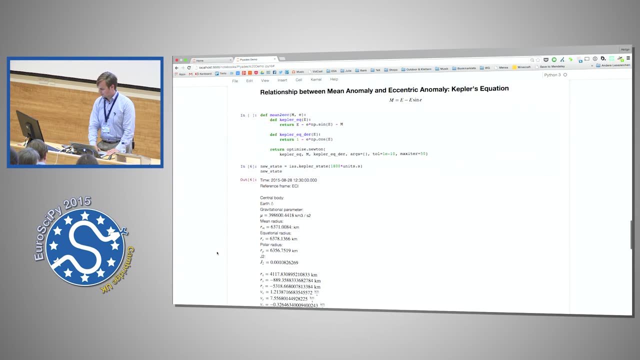 and we get a numerical solution. So half an hour into the future and we get a new state for the ISS. So that's all numbers. And now we want to look at some things. And when you do visualizations, you spend a lot of time setting up figures. 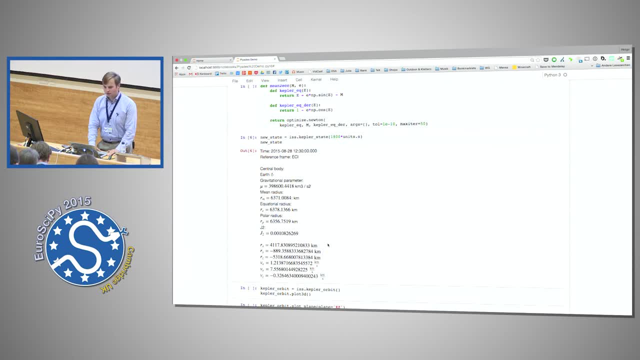 and labeling axes and doing that over and over again And I'm lazy, I don't want to do that. So it's all in my state: vector object And we get this clumsy visualization. So if anybody knows a better way to do 3D lines and surfaces in Python, 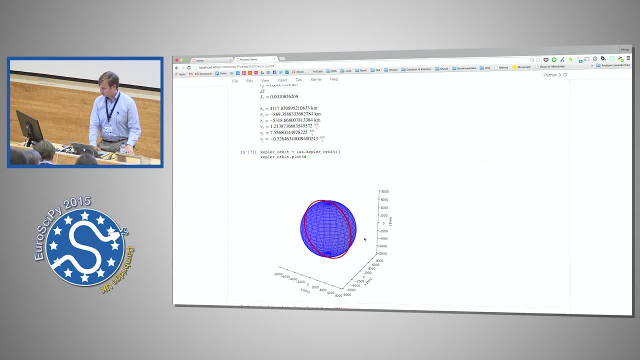 I'll be very glad for suggestions, But instead I'll just do a projection in 2D with Boki and it looks like this. So just to prove that I didn't lie to you, this is the new state And it moved. 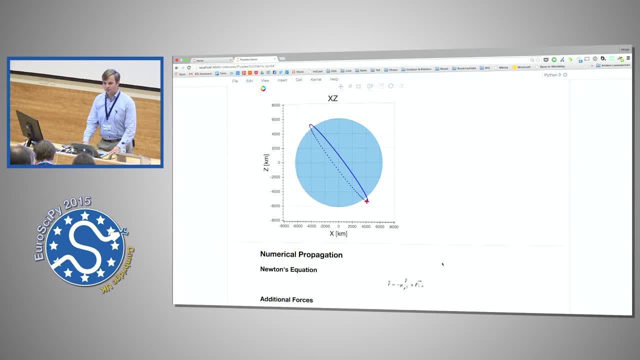 But actually that's only part of the story, because, while this is all idealized, Earth is a sphere and in reality it's not that easy. So in reality we need to do numerical propagation. So what we have here is Newton's equation. 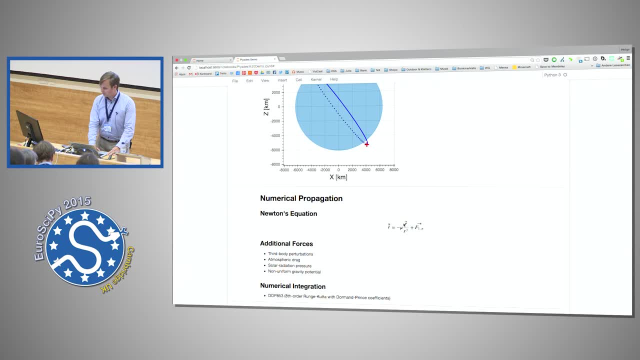 And if you just take this gravity term, it's the same as the simple Kepler case. But we need to add a lot of other forces, so like third-body perturbation, because obviously the Moon and the Sun and all the other planets, they also attract the spacecraft. 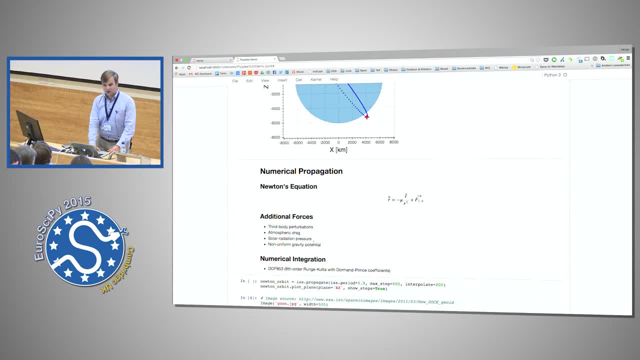 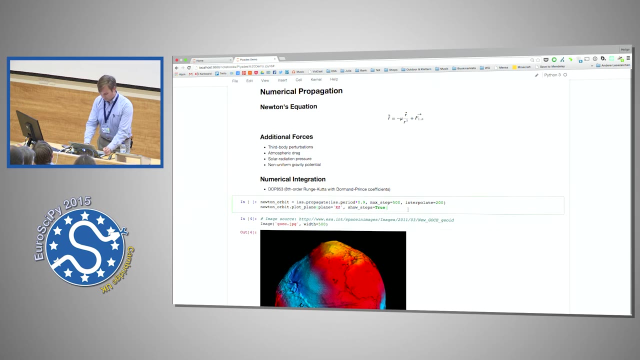 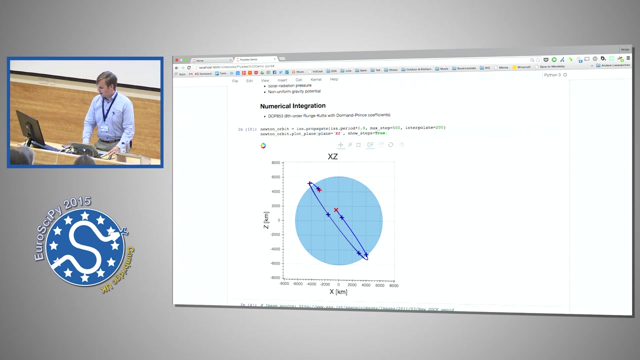 Then there's atmospheric drag- Solar radiation pressure is really important, It plays a role- And of course the non-uniform gravity potential, because the Earth, sadly, is not a sphere. So this is the numerical propagation, And so the blue crosses are the solver steps. 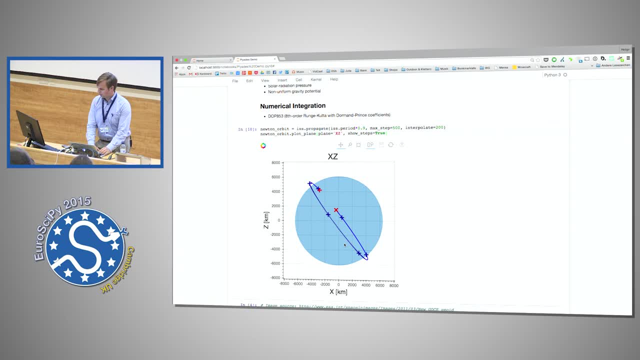 and the rest is interpolation. And it's also quite fast because it's calling us a fortune solver underneath in SciPy. How did you know that this was the correct method for your experiment? Why did you choose your D of O P H? 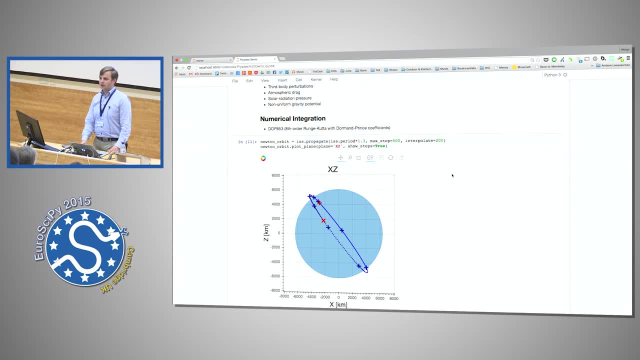 Ah, OK. So the problem is the dynamics of the system is really high. So you have values, So you have For the dynamics. you have six equations and the first three the values are in the thousands, thousands of kilometers. 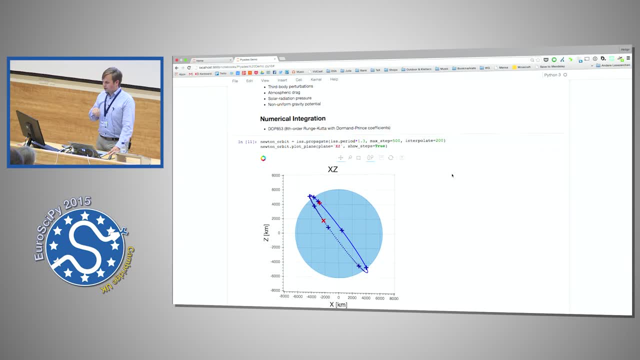 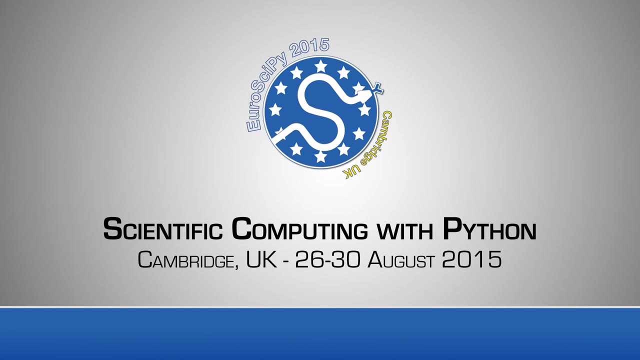 And. But in the velocities you have single-digits kilometers per second, So you need the 8th order Runge-Kutta for that. So in As I said, in reality the gravity potential of the Earth looks more like this lovely potato. 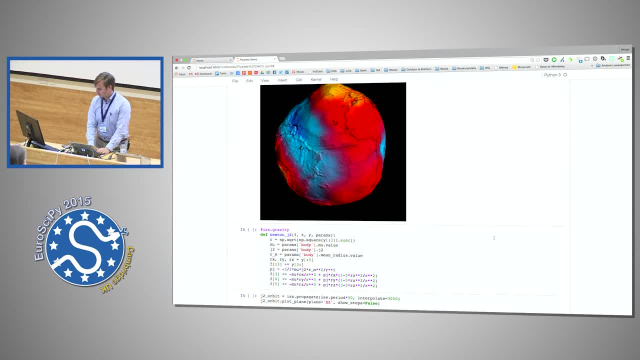 And so we need to refine our force model, And what we do here is we introduce the so-called J2 term And that is Takes into account the oblatness of the Earth so that it looks more like an orange, And I really liked the decorator syntax. 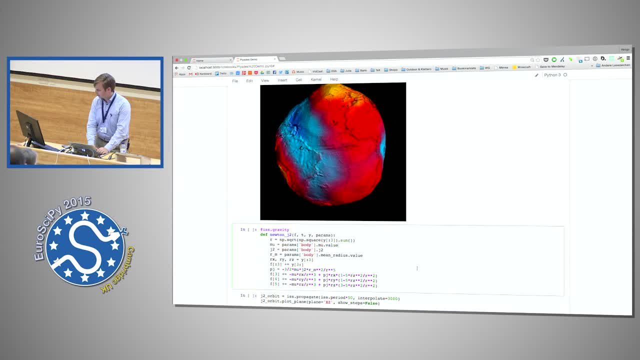 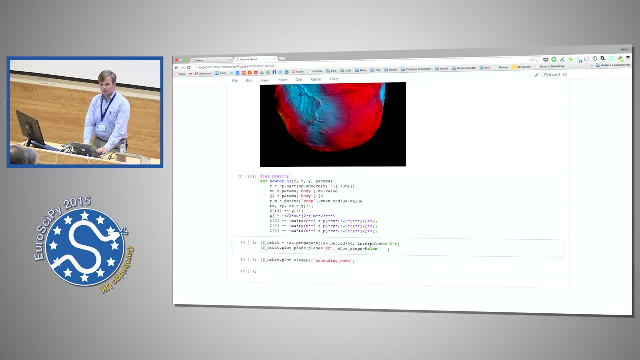 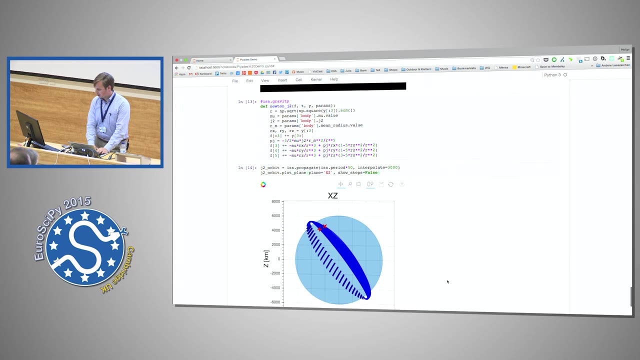 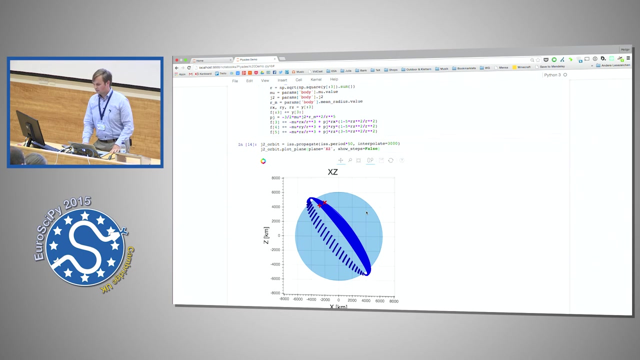 so I can just write my function here and plug it into the integrator like this. And now we do 50 revolutions of the ISS, And again I'm pushing the limits of the visualization. But what we see here is That the orbit is not fixed anymore. 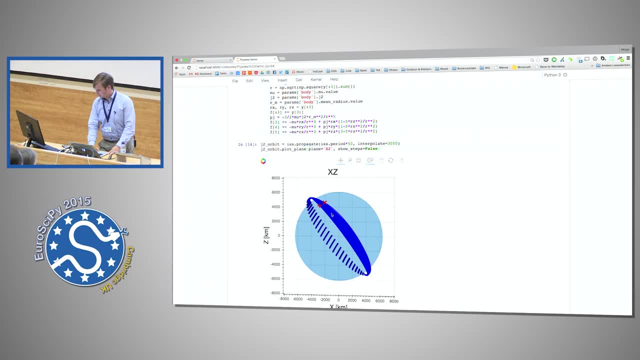 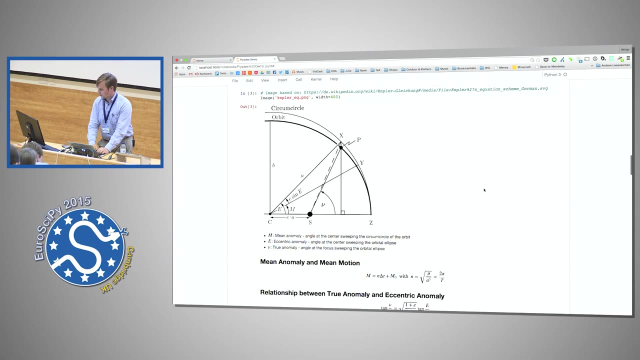 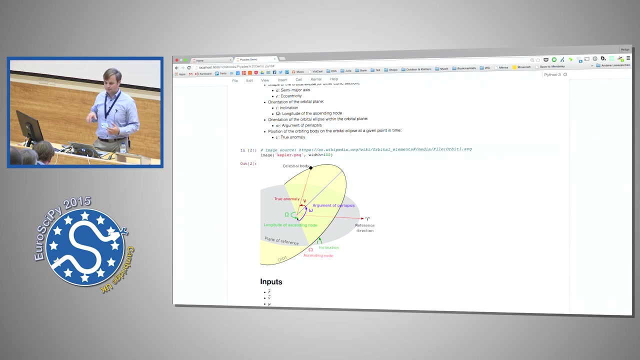 it's moving And It looks like it's turning around in In this direction. So, again, if you think back to the, To the orbital elements, Here The longitude of the ascending node determines the, The orientation of the orbital plane. 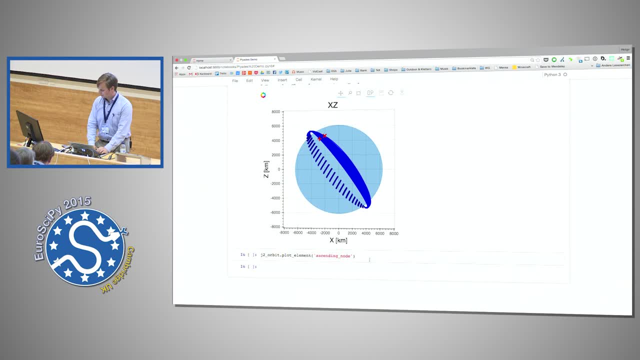 And it seems to move here. So if we Plot this element We see It's decreasing. So, as expected, Any questions So far. If you do the math then you see it And of course we saw it. 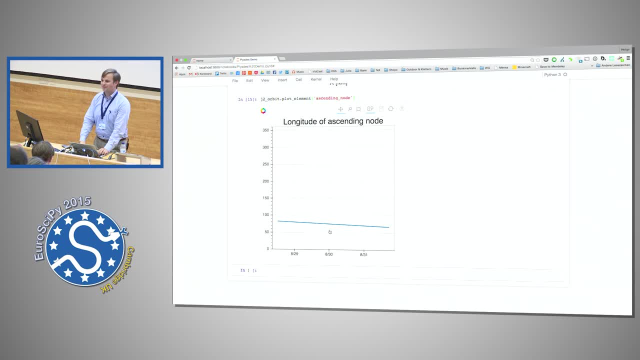 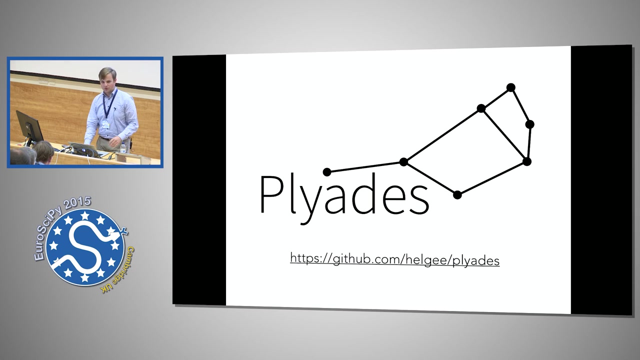 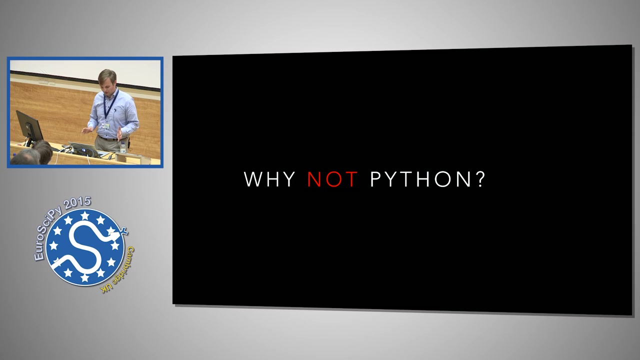 And, of course, we saw it in the visualization. so Where's my cursor There? Okay, so this was a quick Astrodynamics 101. And Now we Talk a little about why not Python? So- and this is best discussed when we talk about the alternatives- 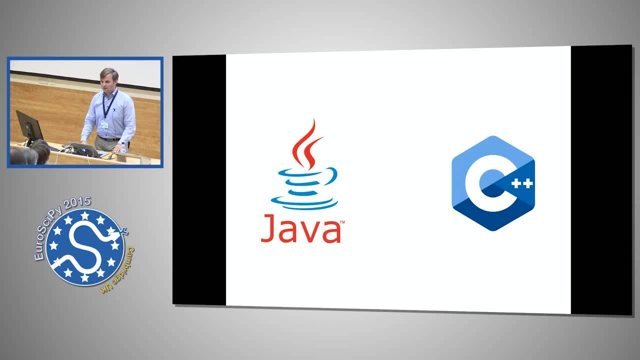 Well, Excuse me, The French space agency, CNES. they're using Java And there's lots of vocal proponents for C++, But in my humble opinion, if we're talking about compiled languages, then nothing beats modern FORTRAN. 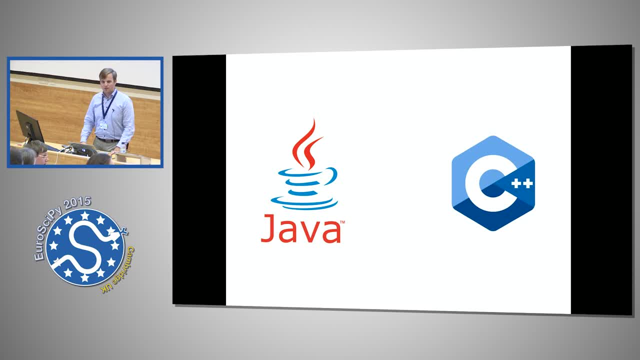 Because a matrix multiplication in modern FORTRAN is just a mud-mull of A And it's not as easy to shoot yourself in the foot as in FORTRAN 77, or C++. And I really don't want to get started with Java. 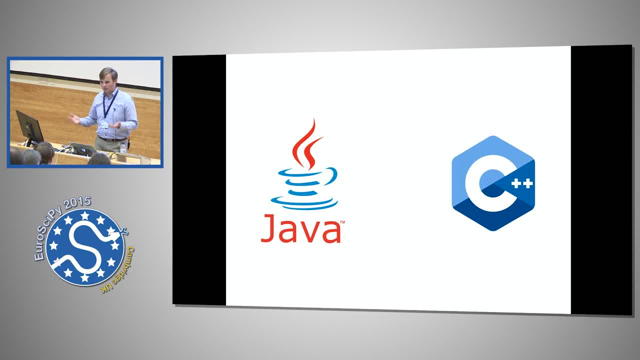 because I don't know how I compile my stuff with AND with MAVEN, with GRADLE, with, And I need Eclipse to even get the methods. So I'm maybe a bit biased here, But I think the real competitor is Julia. 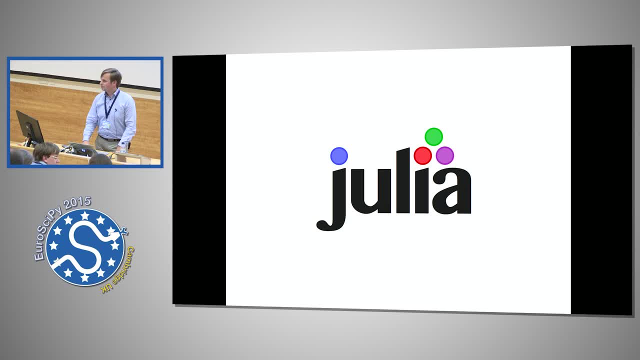 And who of you has tried? Julia, We need those sticky notes So you can see. I don't know if it was a good impression or a bad impression, But I think the language is really well designed and gave me good performance. And what's my main trouble with Python?